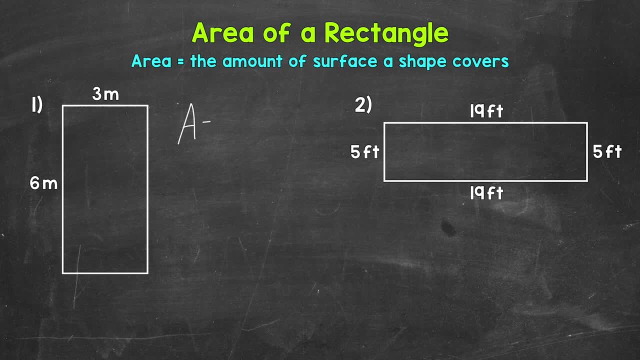 For finding the area of a rectangle, we can use the formula: area equals length times width. I used a cursive L for length, so it doesn't look like a 1.. Not a huge deal though, either way. as long as you know, it's an L when you write out the formula. 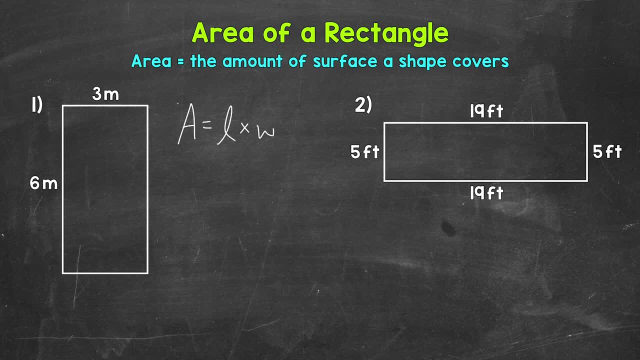 Now all we need to do is plug in the length and width and then multiply. I'm going to use the longer side for the length, so 6 meters, And then 3 meters for the width. So area equals 6 meters times 3 meters. 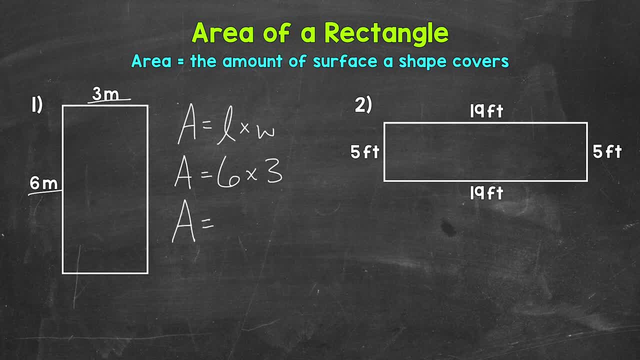 And now we can multiply 6 times 3 gives us an area of 18 square meters. We measure area in square units, so this is square meters. Before we move on to number 2, let's take a look at why we do length times width. 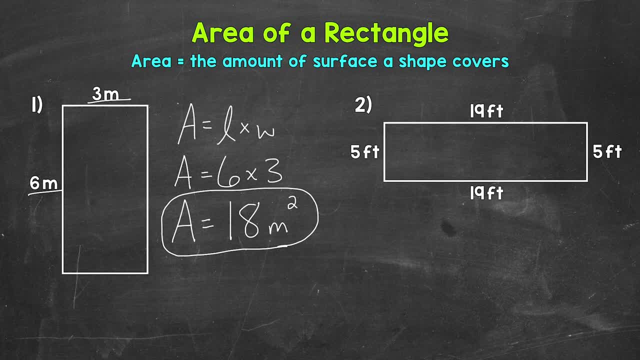 And look at a visual of area. We have 6 meters by 3 meters, So let's draw these out, starting with 6 meters. So I'm going to mark each meter here, so 1, 2,, 3,, 4,, 5, and 6.. 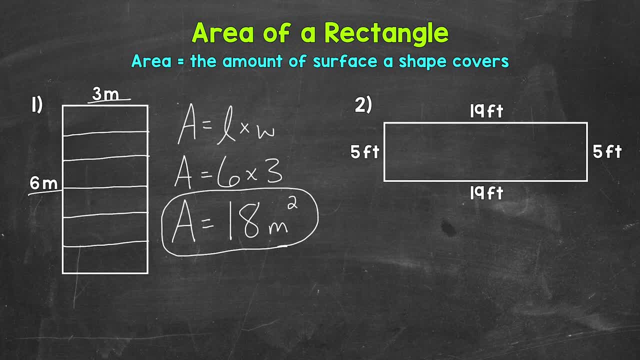 So we have 6 meters there And now we can do the width. so 3 meters: 1., 2, and 3.. You'll notice that we have squares now. These are square units And specifically for number 1,, those are square meters. 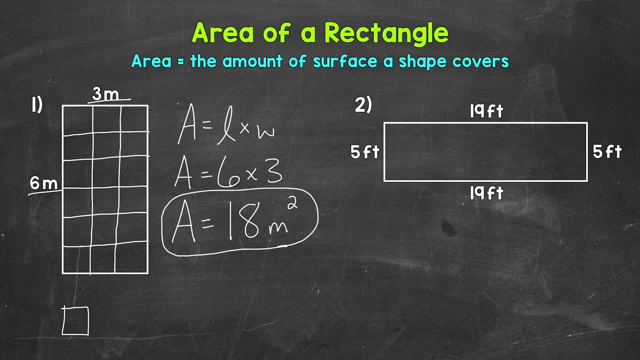 That just means that each square is 1 meter by 1 meter, And this is a square meter. When we find errors, we can use the formula: When we find area, we find how many square units something covers. So for number 1,, how many square meters does this rectangle cover? 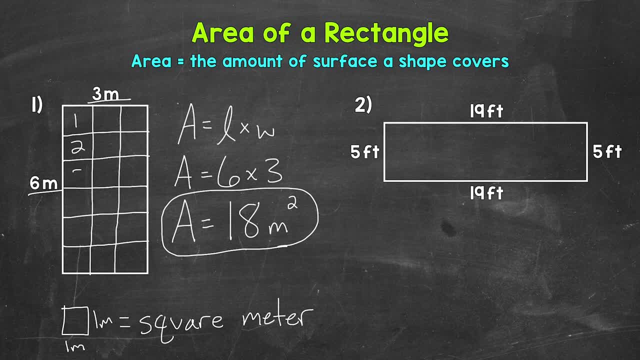 Well, 1,, 2,, 3,, 4,, 5,, 6,, 7,, 8,, 9,, 10,, 11,, 12,, 13,, 14,, 15,, 16,, 17, 18.. 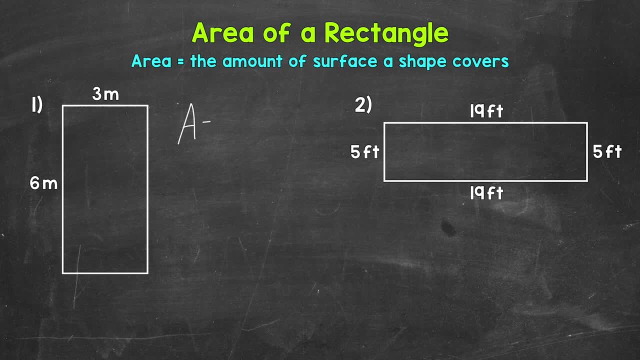 For finding the area of a rectangle, we can use the formula: area equals length times width. I used a cursive L for length, so it doesn't look like a 1.. Not a huge deal though, either way. as long as you know, it's an L when you write out the formula. 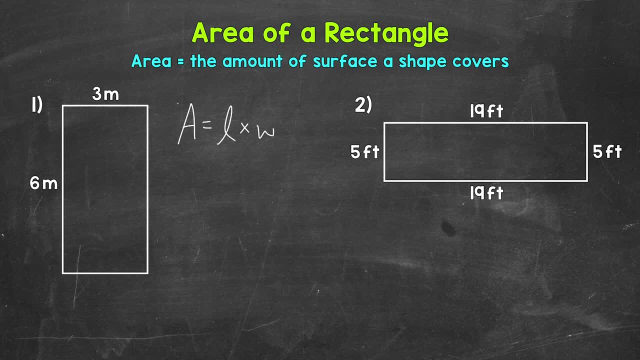 Now all we need to do is plug in the length and width and then multiply. I'm going to use the longer side for the length, so 6 meters, And then 3 meters for the width. So area equals 6 meters times 3 meters. 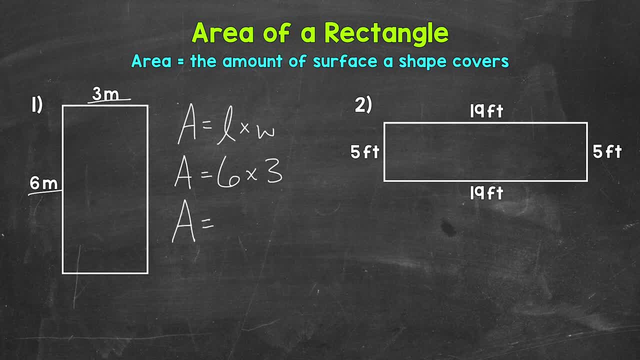 And now we can multiply 6 times 3 gives us an area of 18 square meters. We measure area in square units, so this is square meters. Before we move on to number 2, let's take a look at why we do length times width. 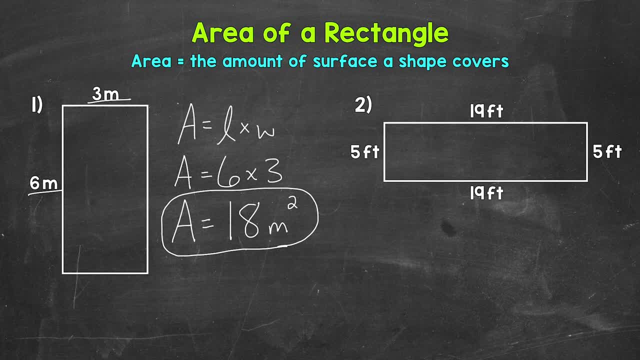 And look at a visual of area. We have 6 meters by 3 meters, So let's draw these out, starting with 6 meters. So I'm going to mark each meter here, so 1, 2,, 3,, 4,, 5, and 6.. 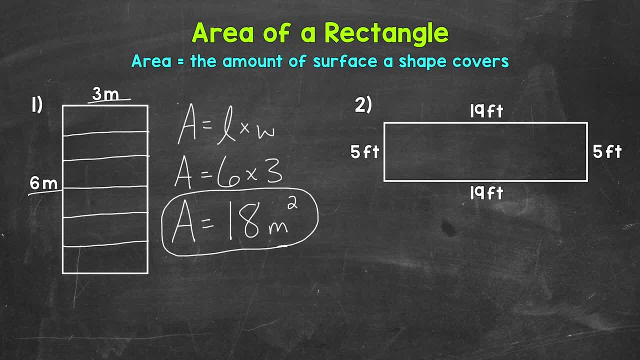 So we have 6 meters there And now we can do the width. so 3 meters: 1., 2, and 3.. You'll notice that we have squares now. These are square units And specifically for number 1,, those are square meters. 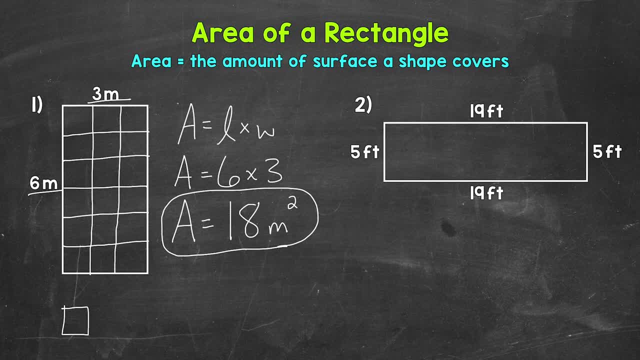 That just means that each square is 1 meter by 1 meter, And this is a square meter. When we find errors, When we find errors, When we find errors, When we find area, we find how many square units something covers. 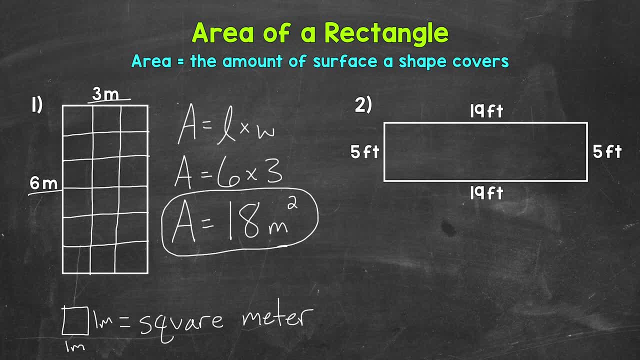 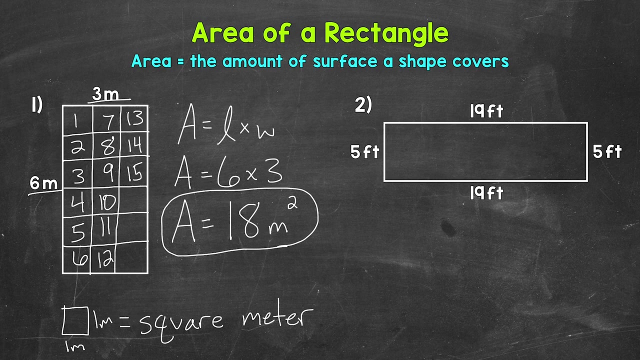 So for number 1,, how many square meters does this rectangle cover? Well, 1, 2,, 3, 4,, 5,, 6,, 7,, 8,, 9,, 10,, 11,, 12,, 13,, 14,, 15,, 16,, 17, 18..